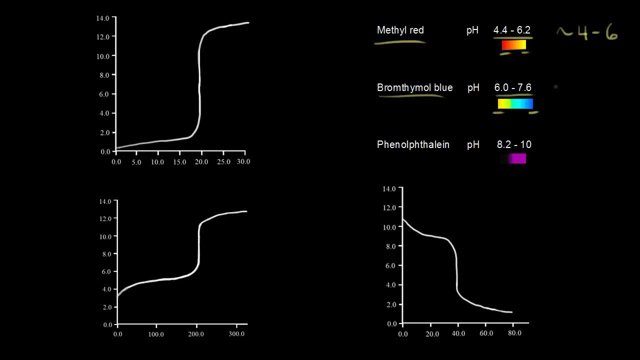 over a pH range of about 6 to 7.6.. So we could say that's approximately 6 to 8.. And phenolphthalein is an indicator that goes from colorless to pink or magenta over a pH range of about 8.2 to 10.. 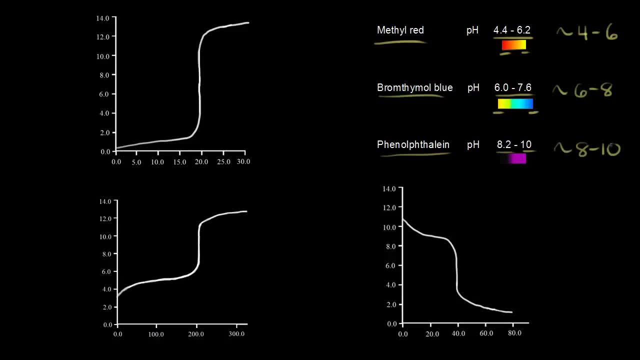 So we could say that's approximately 8 to 10 here. Let's look at our titration curves and let's see which acid-base indicators we could use. All right, we'll start at the top left here. This was the titration curve. 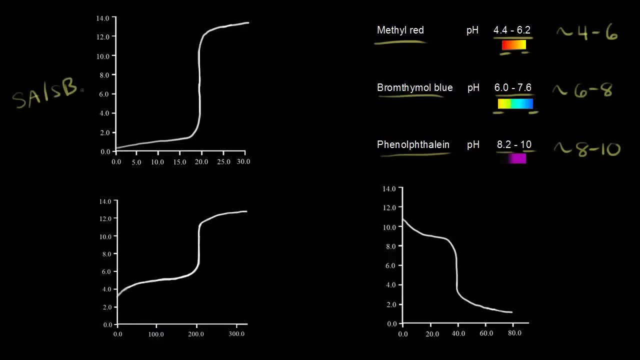 for the titration of the acid base. So we have a strong acid with a strong base, And at the equivalence point the pH is equal to seven. So right, here would be a pH equal to seven, And so this was our equivalence point, right. 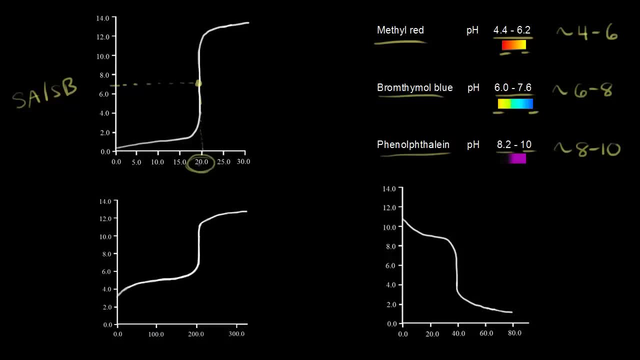 So we drop down here For the example that we did. we did the math: it took 20 milliliters of our strong base to reach the equivalence point. So if you're doing a titration of a strong acid with a strong base, the pH is equal to seven. 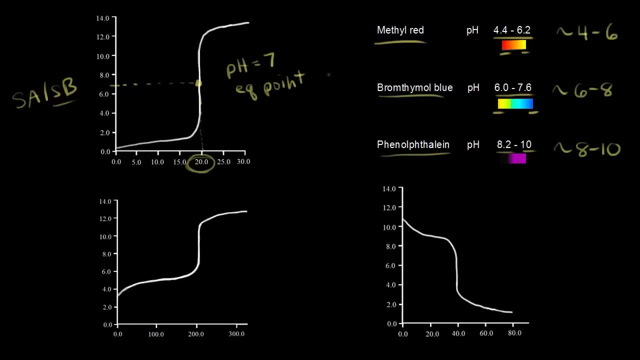 at the equivalence point. All right, so let's think about which acid-base indicator we could use for this titration. You want to choose an indicator that changes color in a range close to your equivalence point. For example, bromothymol blue changes color. 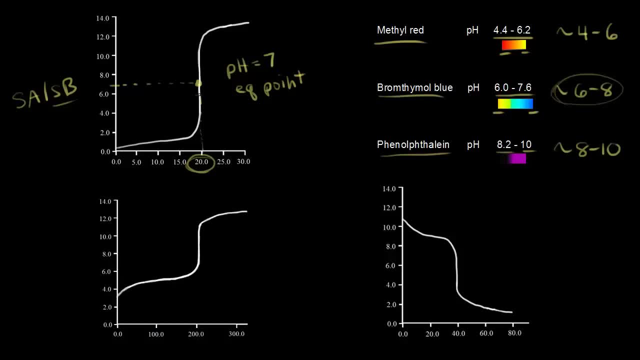 from six to eight right. So, at a pH of six, bromothymol blue is yellow. So right here bromothymol blue would be yellow And then it would change to blue. You might even see some green in there. 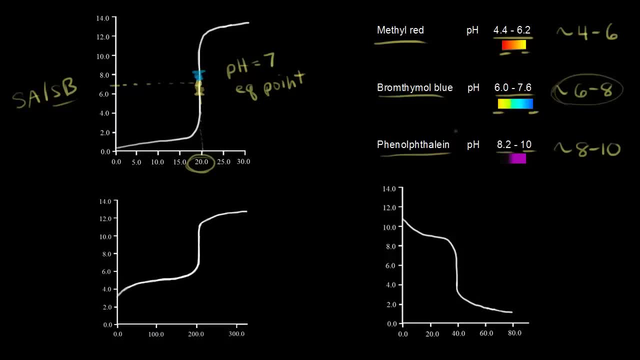 All right. so you see a color change in this range. So bromothymol blue would be a good acid-base indicator to use for your titration. So when the blue color persists, you've reached the endpoint of your titration and you've matched the endpoint of your titration. 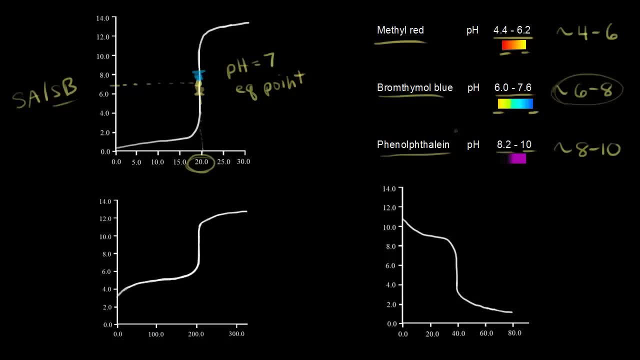 with your equivalence point pretty well. So this is a good way to approximate the equivalence point. For a strong acid, strong base, we have a really steep titration curve right From a pH of about four. let me change colors there. 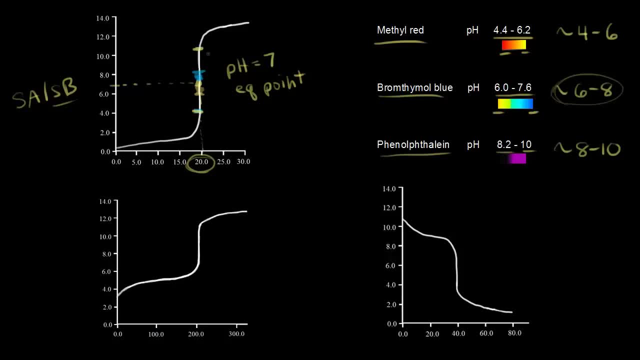 from a pH of about four to a pH of about 10.. So we could've used the other two acid-base indicators too. All right, we could've used methyl red, because methyl red changes from red to yellow in a range of about four to six. 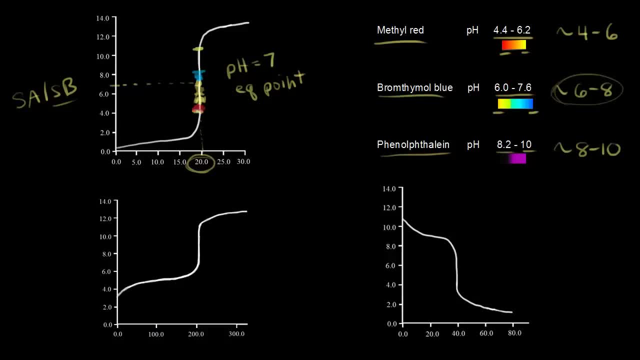 And so that gives you a good approximation of the equivalence point. Or you could've used phenolphthalein, because phenolphthalein changes to magenta right somewhere between eight to 10.. So because you have this really steep titration curve, 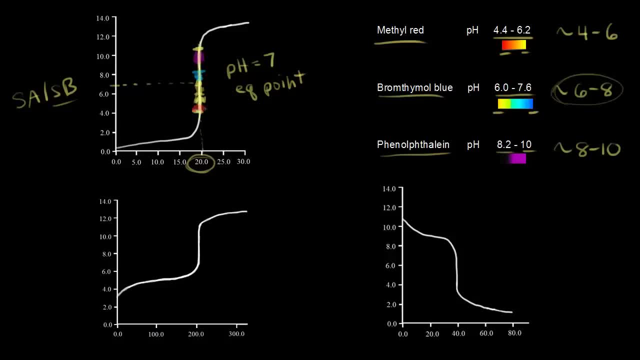 like this: all right, you could've used any of the three acid-base indicators to find the equivalence point for your titration, All right. next let's look at the titration curve for the titration of a weak acid with a strong base. 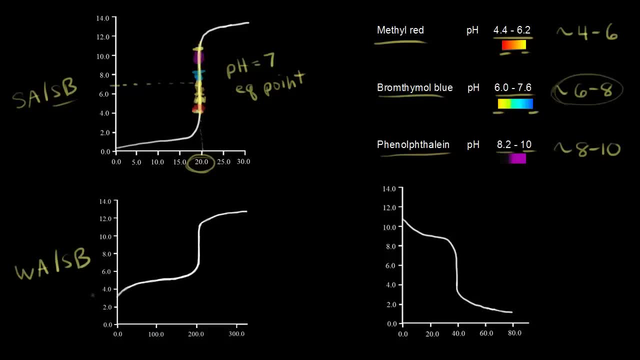 And that was this example over here. So we started with a weak acid. right In our example we used acetic acid, And to the acetic acid we added a strong base, sodium hydroxide. The pH of the equivalence point is greater than seven. 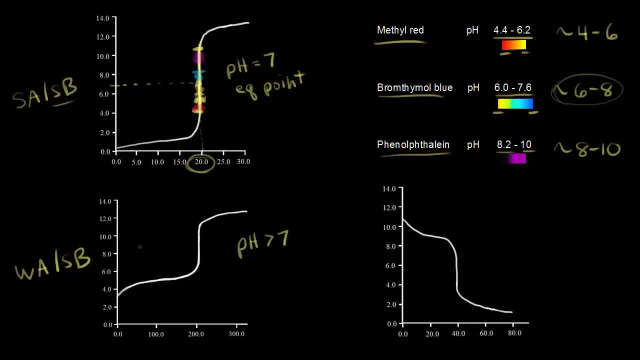 All right, The pH was greater than seven For our example. it was close to nine, right, So it was right about there. just under nine was the pH for our equivalence point, And it took about 200 milliliters of our strong base. 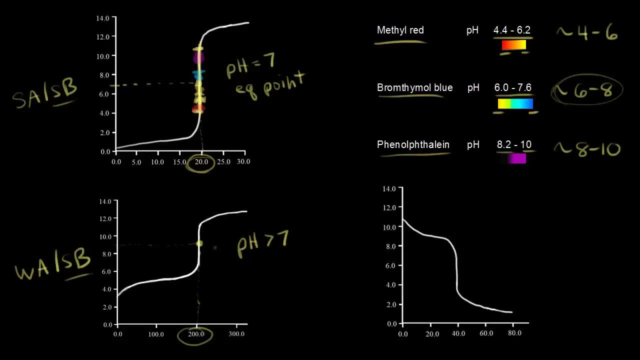 to reach our equivalence point. All right. the reason why the pH is greater than seven at the equivalence point for this kind of titration is when you've neutralized all of your weak acid right, you're left with the conjugate base to the weak acid. 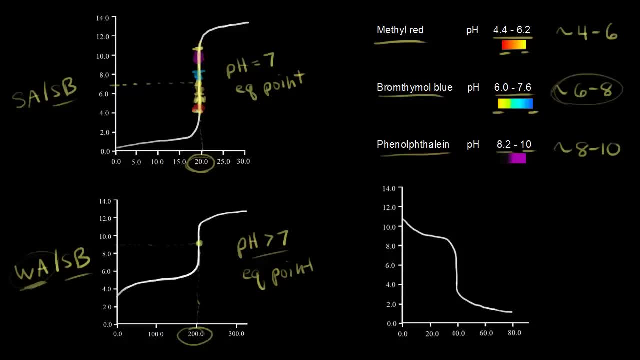 And the conjugate base reacts with water to increase the concentration of hydroxide ions in solution, And that's why your pH is greater than seven. So go back and watch the video for this titration if you want to see the exact calculation. 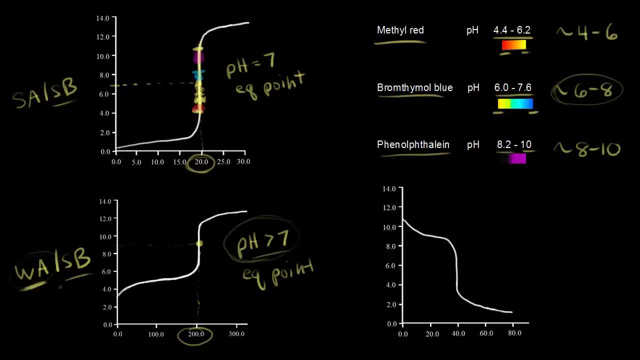 So, for the titration of a weak acid with a strong base, the pH is greater than seven. You want to choose an acid-base indicator that changes color in a range greater than seven, And so, for our example, saline would work really well, because it changes in a range of eight to 10.. 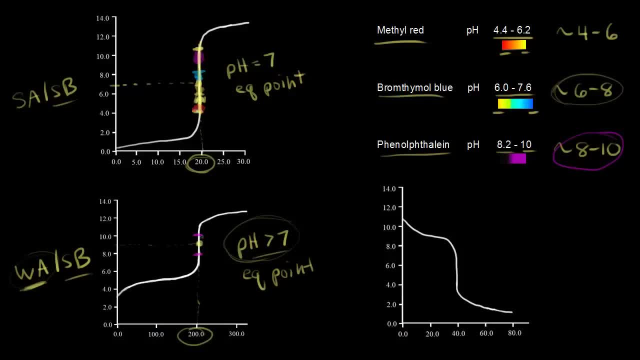 All right. so right in this range right in here, we would see a color change from colorless to pink or magenta. All right, and we would stop our titration at that point, and that's a good approximation of the equivalence point. 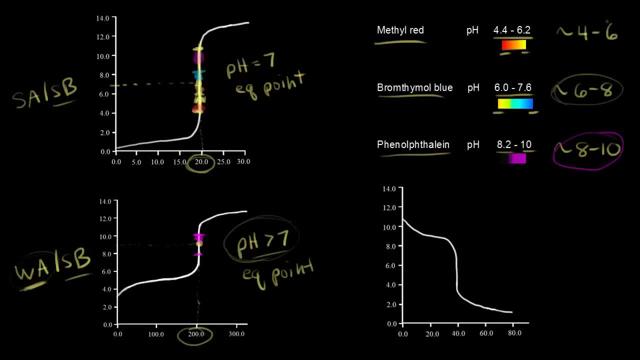 You wouldn't want to use something like methyl red here, because methyl red changes in a range of four to six And you can see four to six would be right in here on our titration curve. So methyl red would be red and then it would change to yellow somewhere in here. 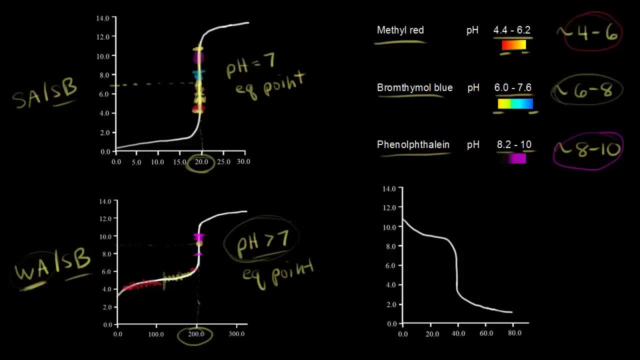 All right. so you get a color change somewhere in here, and so you would miss the equivalence point. This would not be a good acid-base indicator to use, So you couldn't use methyl red here, All right. finally, let's move on to the titration curve. 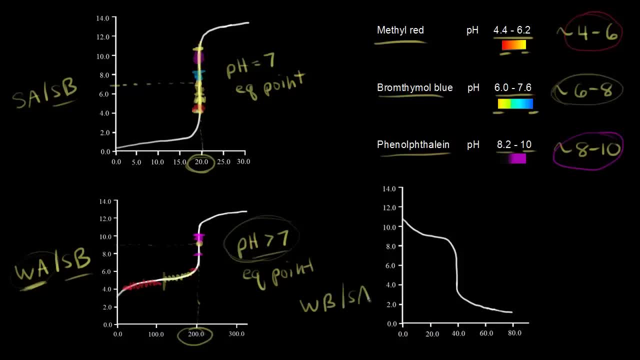 for the titration of a weak base with a strong acid. So we're starting with a weak base and so that's why our pH is in the basic range before we would add in any of our acid here, And in this case the pH at the equivalence point. 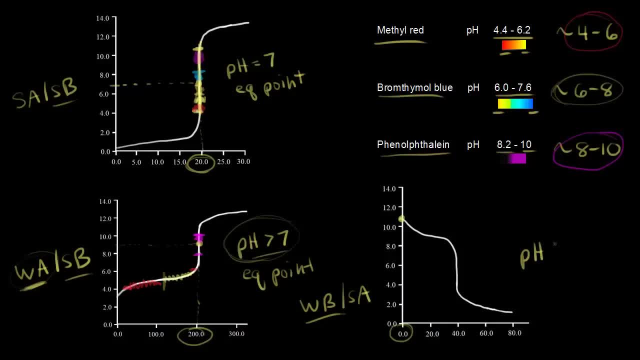 is less than seven. The pH at the equivalence point is less than seven. And that's because if you've reacted all of your weak base with your strong acid, you're protonating your weak base. So in our example, we used NH3, we used ammonia. 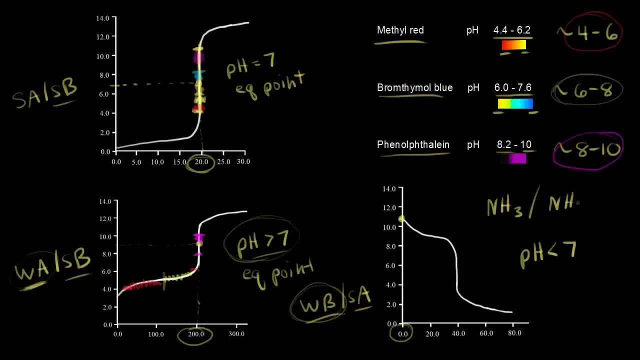 And if you're protonating your weak base, then you're going to be left with NH4+, which is acidic, And so at the equivalence point you have ammonium, Which can donate a proton to water, and so you increase the concentration of hydronium ions in solution. 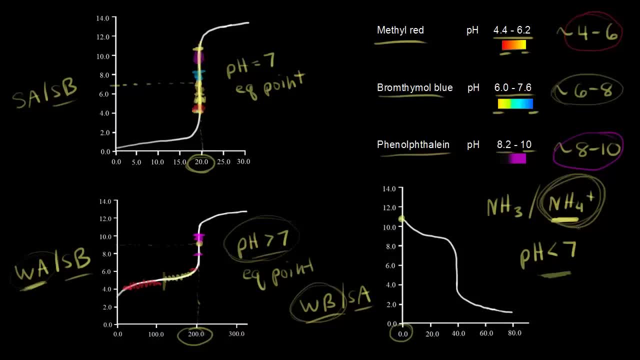 And so at the equivalence point, the pH is less than seven. Once again, watch these videos if you want to see the exact calculation for that. So your pH is going to be less than seven. In our example, we got a little bit over five. 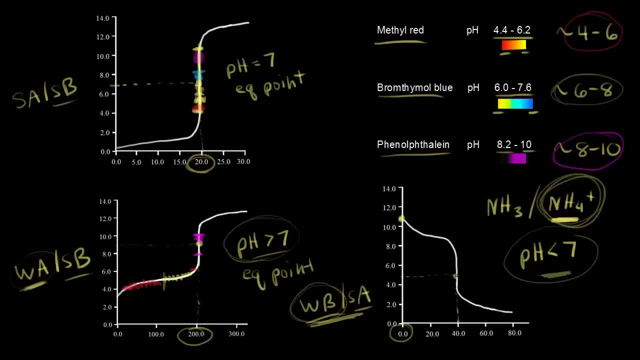 So right about there would be the equivalence point. So if you're thinking about, which acid-base indicator do you want to use? you want to use one that changes color at a pH less than seven, So methyl red would be a really good one to use here.